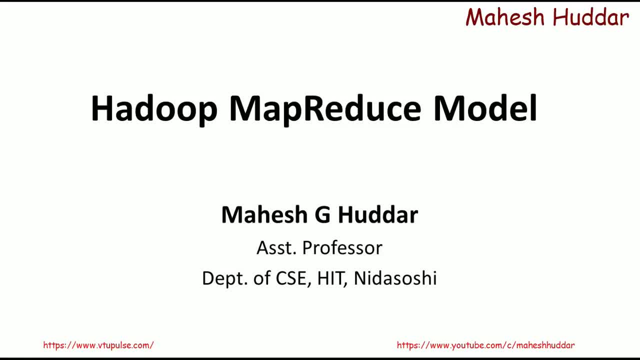 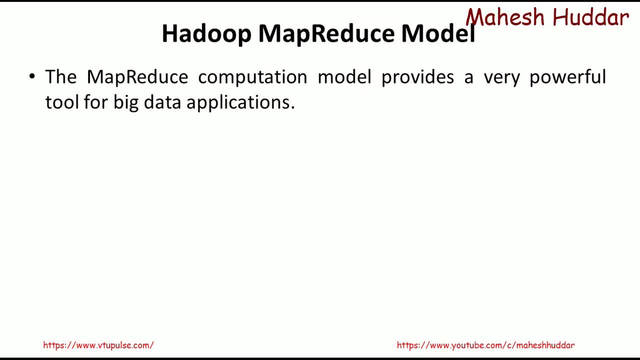 In this video, I will discuss Hadoop MapReduce model. The MapReduce computation model provides a very powerful tool for big data applications. Whenever there is a need to process a large amount of data, MapReduce model can be used and it works very efficiently to process a large amount of data. 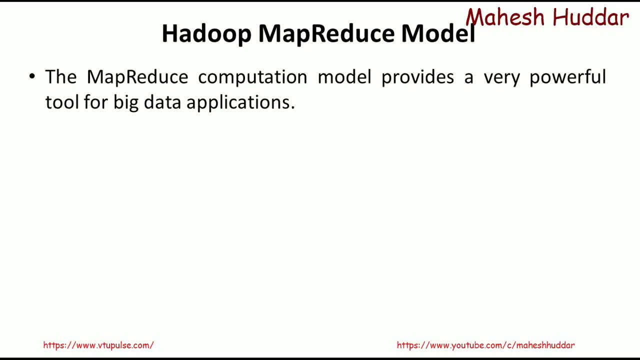 Its underlying idea is very simple. There are two stages in Hadoop MapReduce model. The first stage is the mapping stage and the second stage is reducing stage. When I say two stages, these are the important stages of MapReduce model. Along with these two stages, there were some other stages like splitting data. 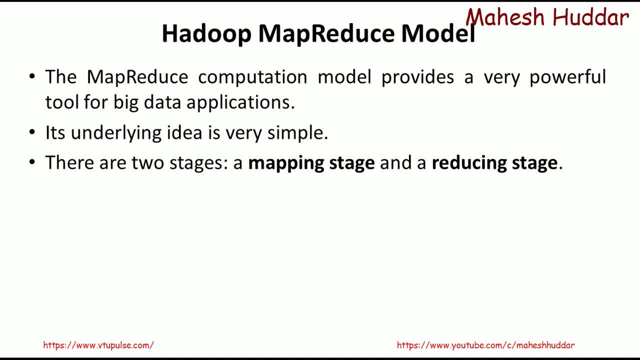 combiner stage, shuffle stage, so that it will become a complete Hadoop MapReduce model. So to understand the basic principle, we will see these two stages first. Later we will see the remaining stages. In the mapping stage, the mapping procedure is applied to input data. 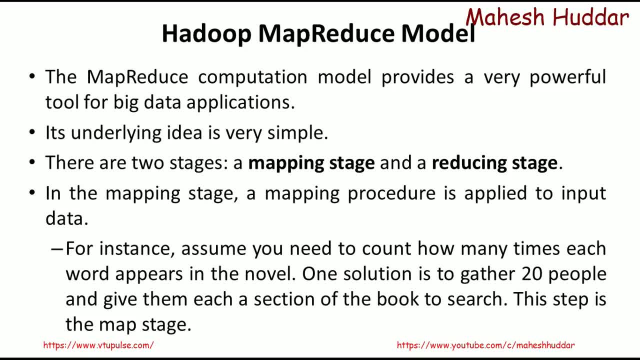 So there is a procedure or you can say that the program is applied to input data. Now, for instance, let us say that you want to count how many number of times each word appears in a novel. There is a big novel and you want to count how many number of times each word appears. 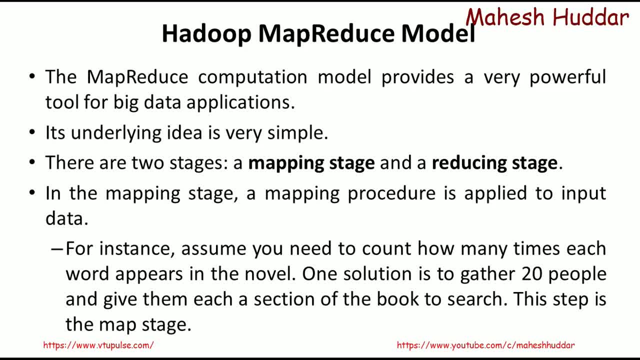 in that novel. Now, let us say that if one person is counting how many number of times a word appears, let us say that it takes 10 hours to complete that task. Now, if that particular task is divided among two people, definitely the amount of time required to count how many. 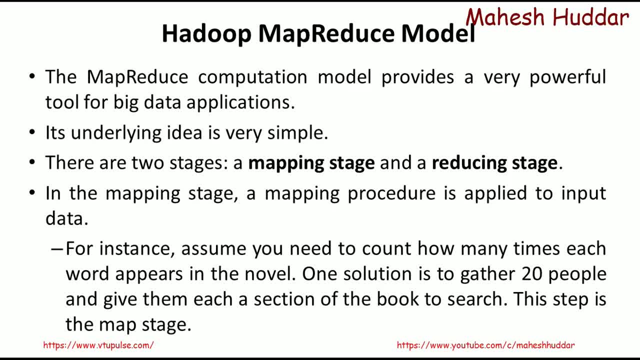 number of time each word appears in the novel is definitely 5 hours. If the same thing is divided among 20 people, it will be half an hour. So this is the underlying principle of MapReduce model: Rather than doing the task by a single person, divide that particular. 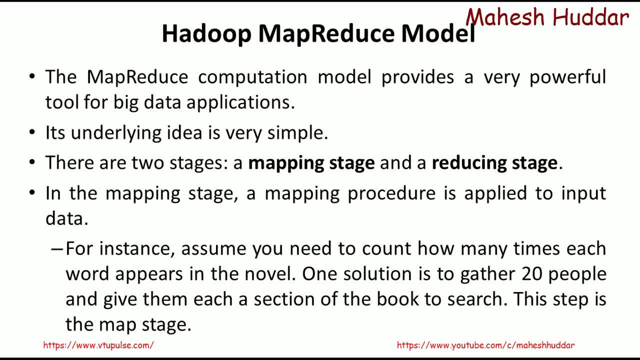 task among number of people so that we can reduce the amount of time it takes to process the data. So in mapping stage the data will be divided among different data nodes. That data nodes will be assigned some task. They will do that particular task. The result: 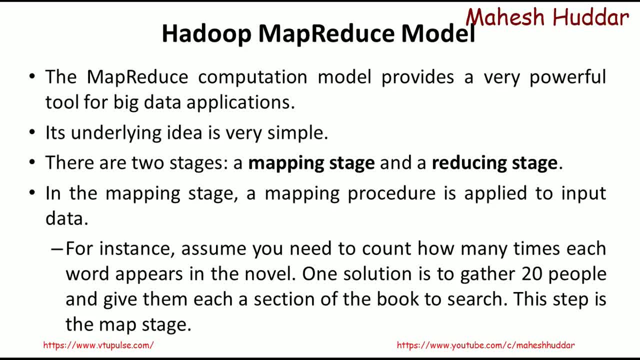 will be given to the reducer step. So what is the reducer step will do? It will take that particular result and then it will aggregate that particular result. So to understand in detail, we will take a very small text file. Let us say that the text file contains: 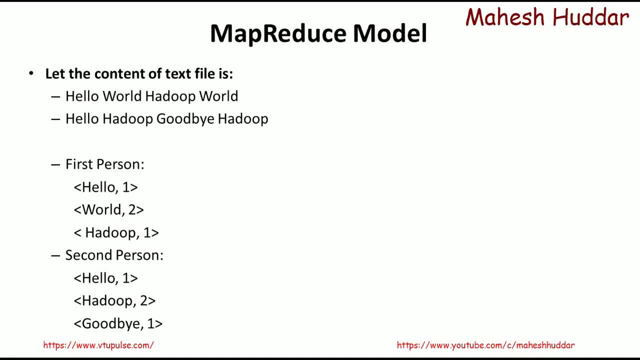 some data. So we will take a very small text file. Let us say that the text file contains two lines. The first line is hello world, Hadoop world. The second line contains hello Hadoop, goodbye Hadoop. So there are totally two lines. are there in this case, And what? 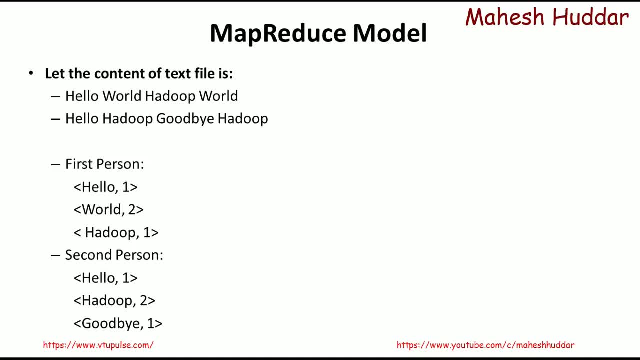 we do over here is we will assign the first line to the first person to count how many number of time each word appears, And we will assign the second word line to the second person so that he can count how many number of times each word appears. 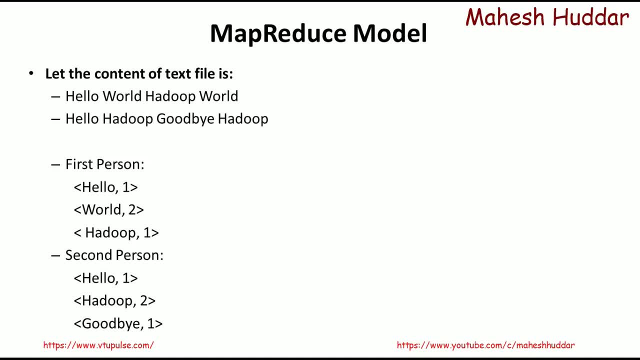 Now, this is the task we have assigned to each person. So there are two persons. One line is assigned to first person, The second line is assigned to second person. So what is the task? He has to count how many number of time a particular word appears in that. 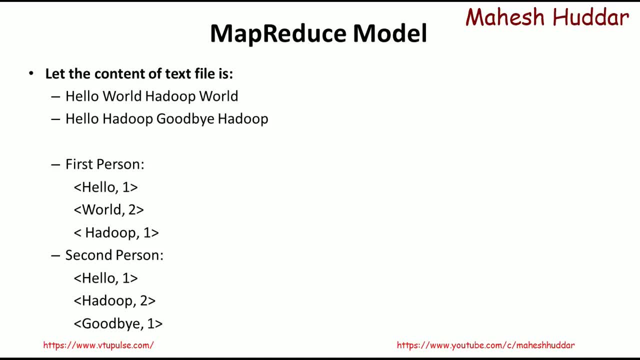 line. So that is what his task, So what that person does is: he will go through that particular line, He will see how many number of times each word appears And he will create a first person's output. So he will create a first person's output And we will create. 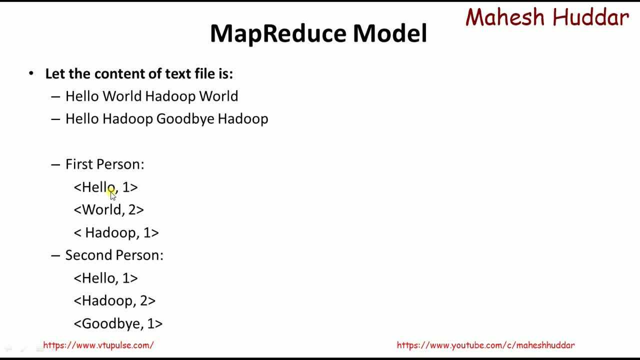 a second person's output. So we can say that the output will be in the form of key and value pair. The key will be the word and value will be how many number of times that word appears. So if you see the first person's output, 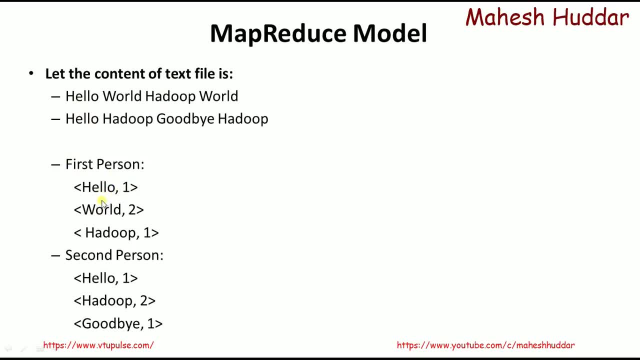 the first person says that hello world appears one number of time. world appears two number of times And Hadoop appears one number of time. What the second person is saying Hello by is appearing one number of time. now, once the result is available from both the persons, 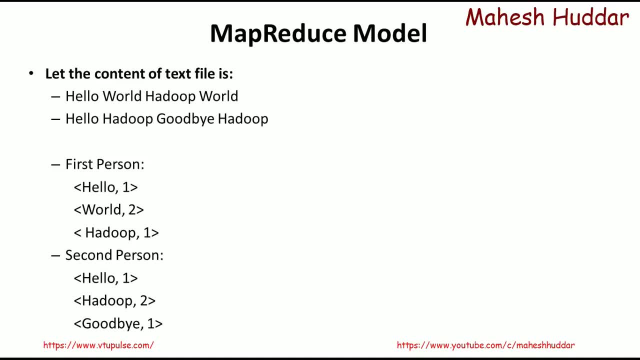 this result can be aggregated by the reducer. so what the reducer will do. reducer will ask each person: give me the word and along with what is the value. so the first person say that hello is appearing one number of time. what the second person says: hello is appearing. 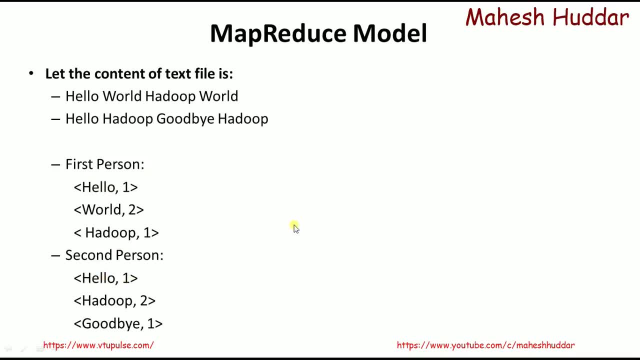 one number of time. the reducer will add, because the keys are same. he will take create one more output file where hello will be the key and value will be one plus one, two in this case, and the first person says that world is appearing two number of time. the second 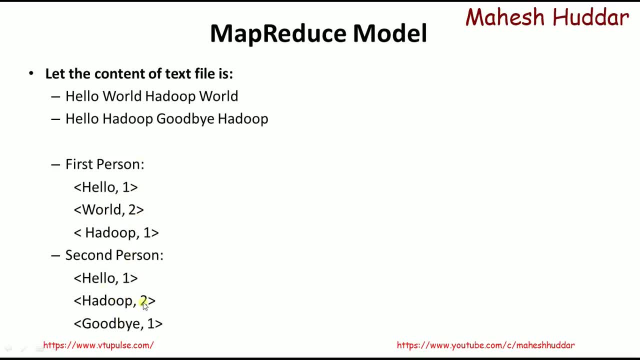 person says that there is no world, he will create one more output file where world will be the key and two will be the value. in that case, the first person says that hadoop is appearing one number of time. the second person says that it is appearing two number of time. 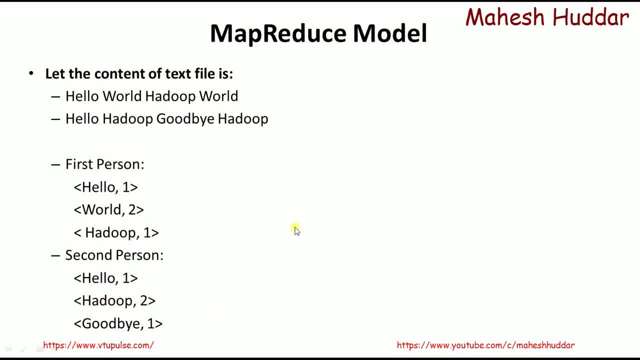 the reducer will create one more output file, that is, hadoop is the key and three will be the output, because one plus two is three is the answer. in this case, the first person says there are no words in in in file and the second person says that there is a goodbye word and it appears one time. 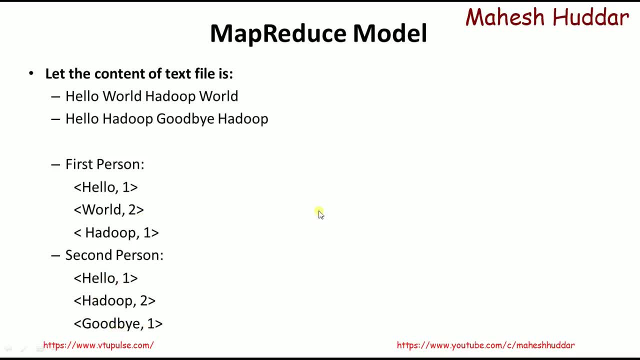 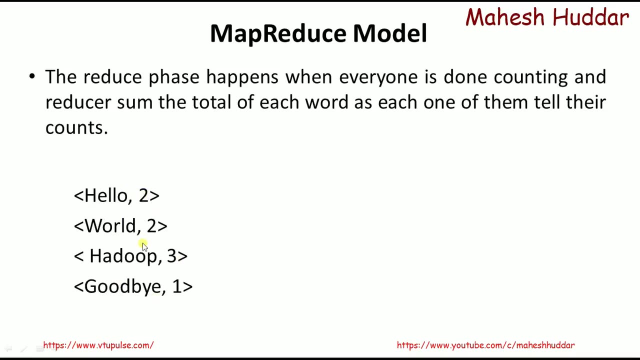 another output file will be created with goodbye is the key, and one will be the output. that is how actually the reducer will do. it will aggregate the result from the mapping the stage. this is how actually the output looks like. so this is the basic underlying idea behind the map: reduce model. 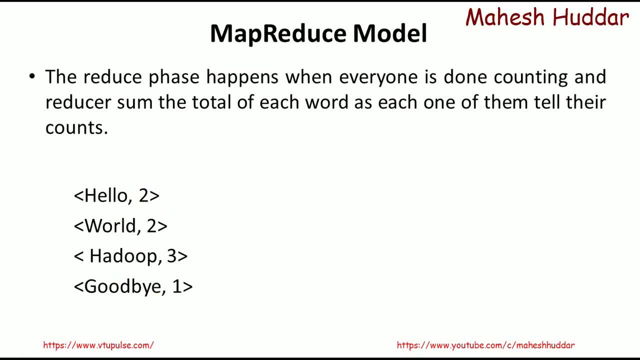 so what happens in map reduce model is the task will be divided among different machines. the each and every machine will do the task and the result of the each machine will be aggregated by the reducer model. so that is what the underlying principle in map reduce model. so, as i said earlier, map reduce model has actually five steps, not two steps. that 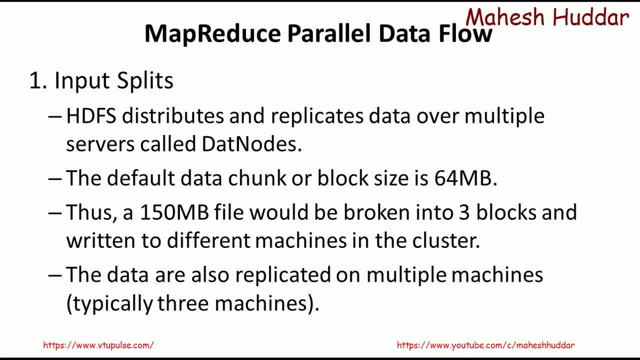 is a mapping stage and reducing step. so we will try to understand each and every step, their functionalities and whether they are compulsory steps or they are optional steps. so that is what we will try to understand now. what is the first step is there is something called as input split. what is the input split is whenever a data, whenever a client wants. 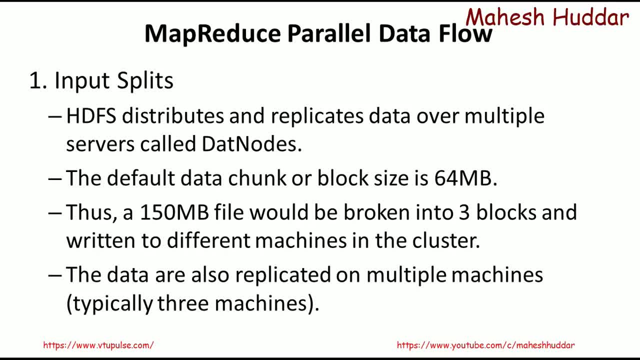 to write some data into the hadoop cluster- hdfs cluster. the data will be divided into blocks. ah, it is called hdfs cluster. the data will be divided into blocks. it is called hdfs cluster. it is also called as a chunk. the size of the block is 64 mb and this particular block of 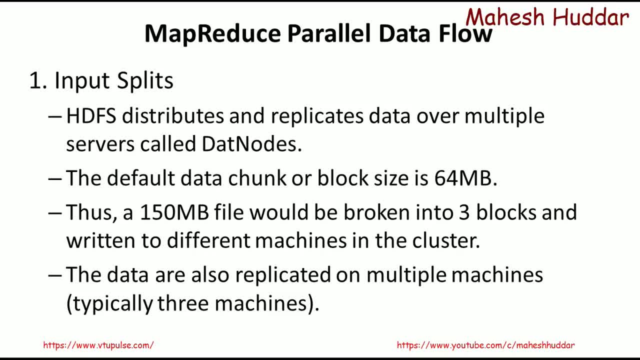 information will be written into data nodes. let us say that a client wants to write 150 mb of data. in that case, the data will be divided into three blocks: the first block size is 64 mb, the second block size is 64 mb and the third block size is 22 mb, 64 plus 64 plus. 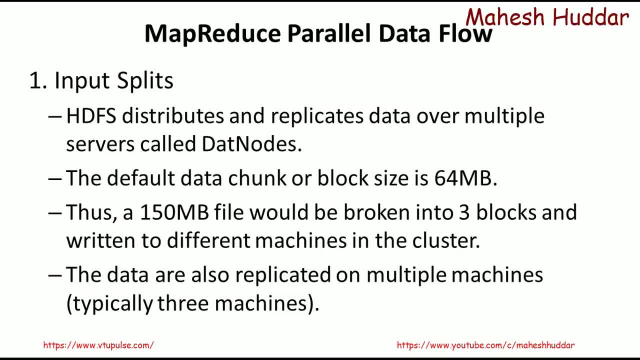 22, which is equivalent to 150 mb. all these particular blocks will be written on different data nodes at the same time. these particular data blocks are replicated on different data nodes. the replication is done to safeguard from any failures in the system. for example, if any data node fails, the data should not. 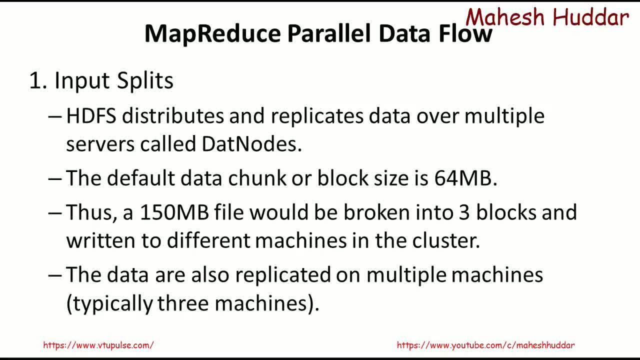 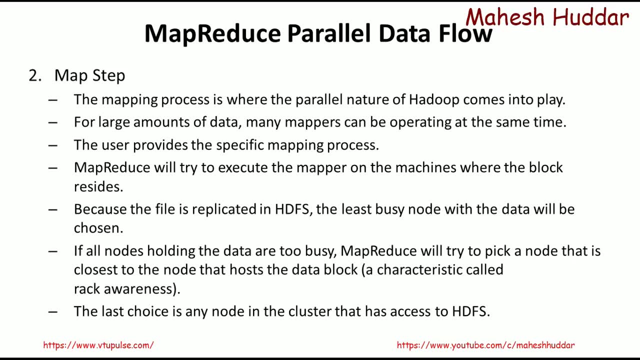 be lost if it is replicated on different data nodes. the data will be available for client to process in that case. so this is the first step. So this is the first step of Hadoop MapReduce model. the second step is actually the map step. what the map step does is the data is divided into multiple number of blocks and 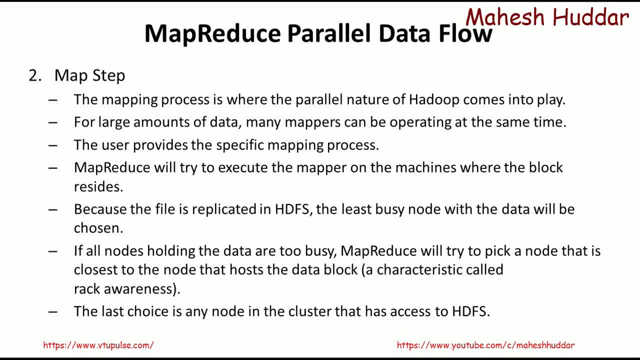 that particular blocks of information is stored on different data nodes. now what happens here is, whenever a client wants to do some processing on that particular data, the mapping or you can say that the actual processing will takes place on the data node where the data is actually present. in the previous case, the data was divided into three data, three data blocks. 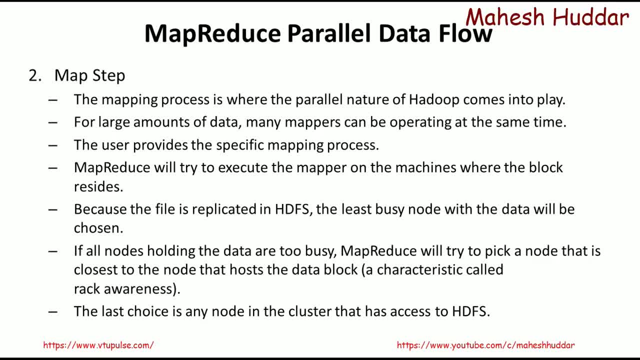 so they must be available on three data nodes. the processing will takes place on three different data nodes. so that is what the mapping process is. rather than doing the processing on one machine, do it on three machines. so definitely the time taken on three machines will be less. 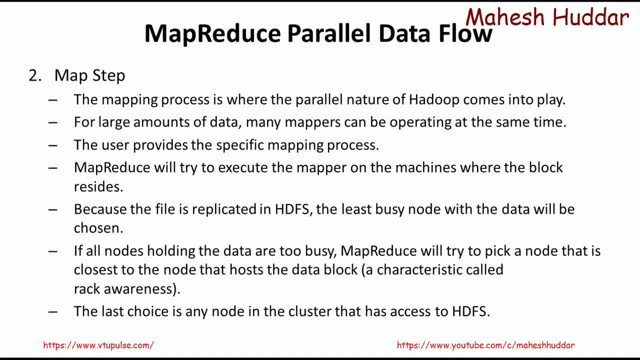 than the time taken on the machine. one machine and the result of three machines can be aggregated in the further steps. So that is what actually happens. But in mapping step the one question comes in front of us is: the data blocks are replicated. For example, if there are more than eight data nodes are there in the HDFS. 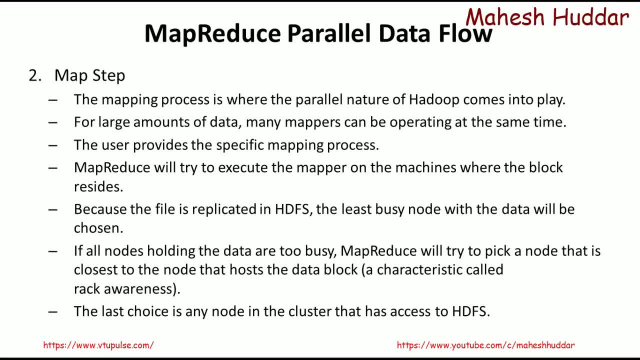 cluster. one data block is replicated three times, So the data block is maybe present on one data node. the same data block may be present on different data nodes. Now where the processing should happen, processing should happen only on one data node, it should not happen on all the. 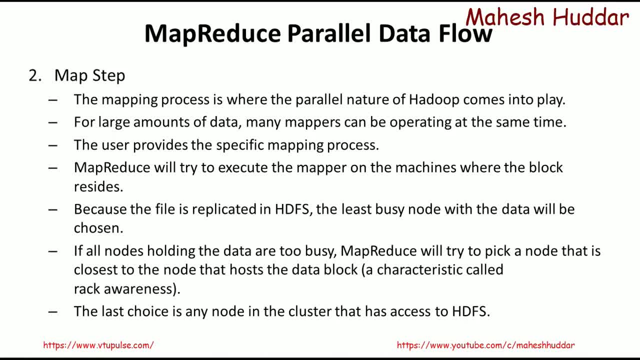 data nodes where the same data is present. For example, the block in block one is present on data node one and data node two. the processing on data node block of information one should take place only on data node one or data node two. it should not happen on both the cases. If data block 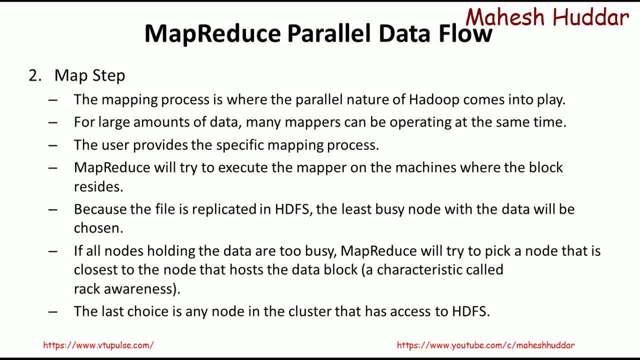 two is present on data node three and data node two, it should not happen on both the cases. If data block two is present on data node four, either the processing should take place on data node two or three, because the same information is present on both the data nodes. So because there, 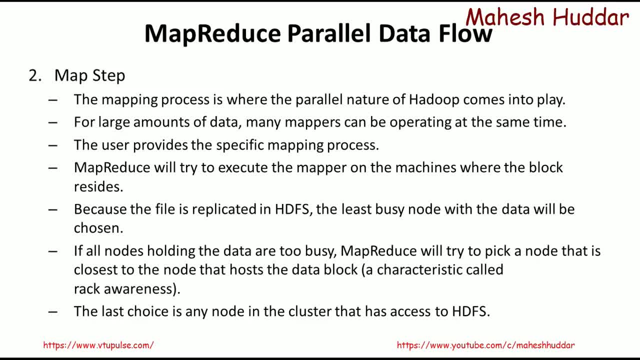 is a replication, the mapping step, or can say that the mapper has to identify where the where the processing should take place. So what HDFS does is, or can say that the MapReduce model does, is it will choose the least busy node. 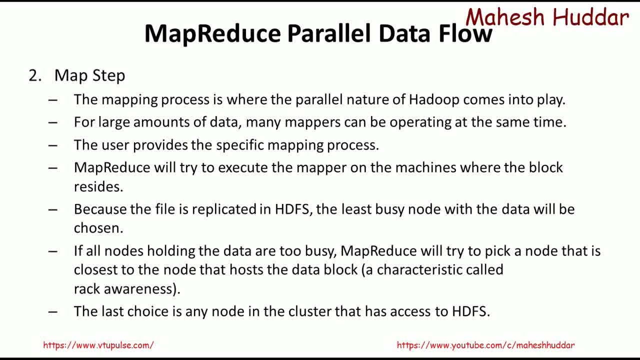 For example, data block one, data block two, data block three, data block three, data block four. data block one is present on data node one and data node two. data node one is more busier compared to data node two. In that case, the MapReduce model selects the second data node because it is less busier. 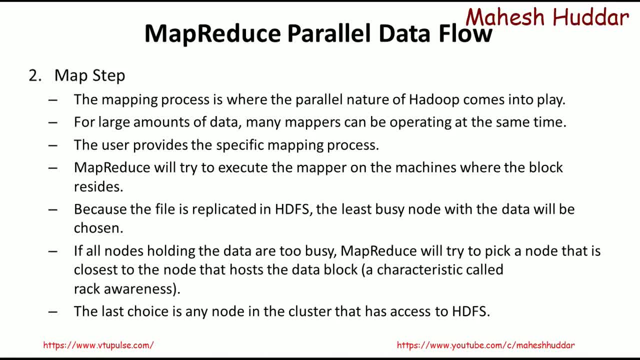 compared to the first data node. Anyhow, the data is present on both the nodes. the second one is less busy, So select that particular node for processing. So that is the one possibility. The second possibility is, if both of them are busy, now what what I supposed to do In that case? select. 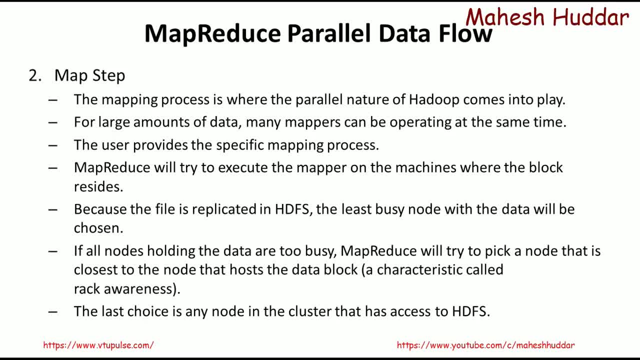 the one which is nearest to the client. For example, as we have discussed in the earlier case, there is something called as data nodes are arranged in the form of racks. One set of data nodes may be present in one location, another set of data nodes may be present in another location. So whenever all the data 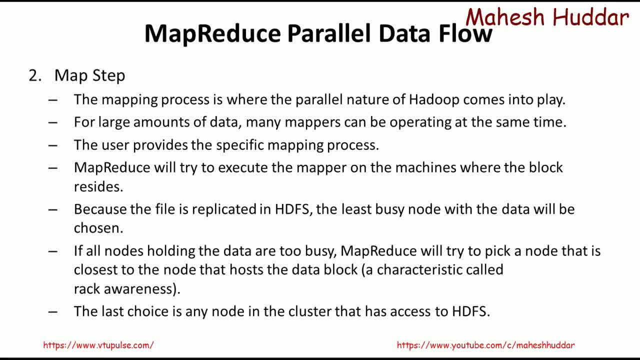 nodes are busy, the one which is nearest to the client. that can be given, that can be used for processing. So that is the second possibility. The third possibility was is select any node in the cluster for processing purpose. So that is the second thing. So what happens in the first step? the data. 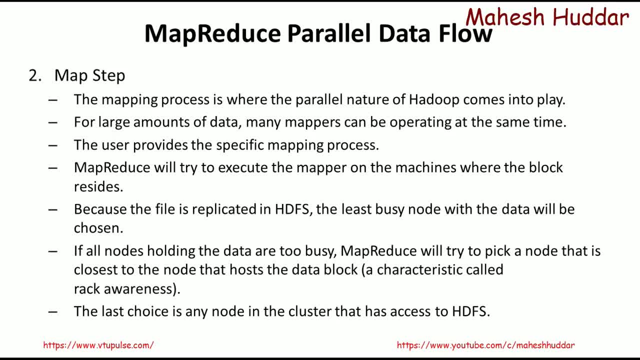 will be divided into data blocks. those particular data blocks will be stored on a different machines as well as they will be replicated on different machines, that is, data nodes. What happens in mapping step is: the actual processing takes place in the mapping step Here, because the data is 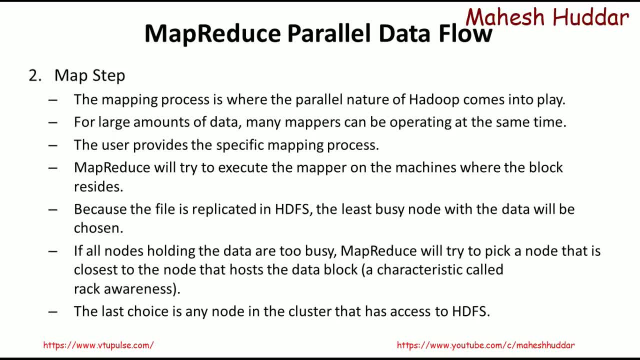 available on multiple number of machines. because of the replication, the processing will take place on one of the machines where the data is available. So if three data blocks are there, the processing will take place on three data nodes and the result will be passed to the next step. So what will be the result? in word count program, The result will be: 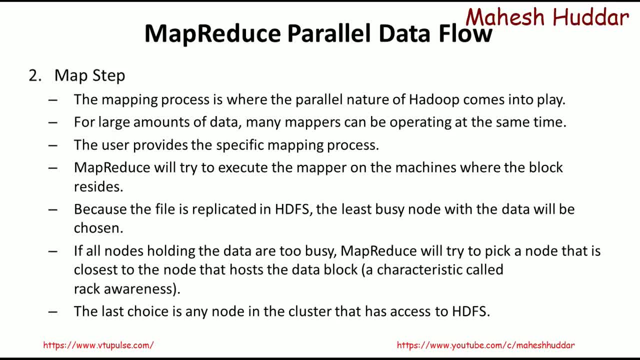 a result in the word count program is that is, word count program means counting the number of times each word appears. So what is the output? the word, that is the word, as well as what is the number of of times the word appears in that particular data node. So that is what the output, So that will be. 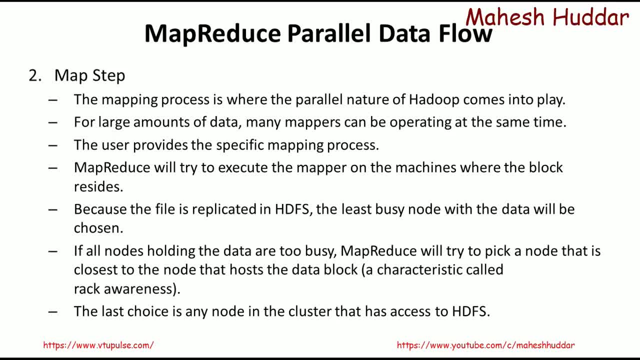 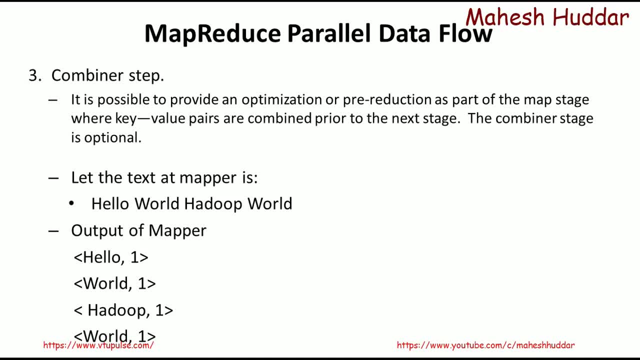 the output to the next stage. So the next stage is something called as a combiner stage or a combiner step. What happens in this case is the combiner step takes the key value pair from the previous step and then it will combine the result depending on the keys. For example, I will take: 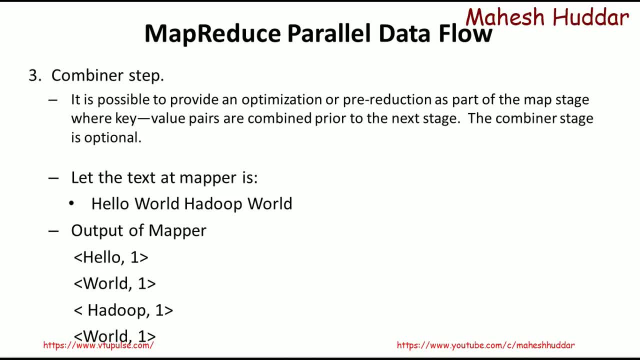 one example in this case. Let us say that the text file is hello, world, Hadoop and world, and the output of mapper is actually what mapper does is. it will count how many number of times it will create an output file consisting of the word and its value. For example, hello is appearing one. 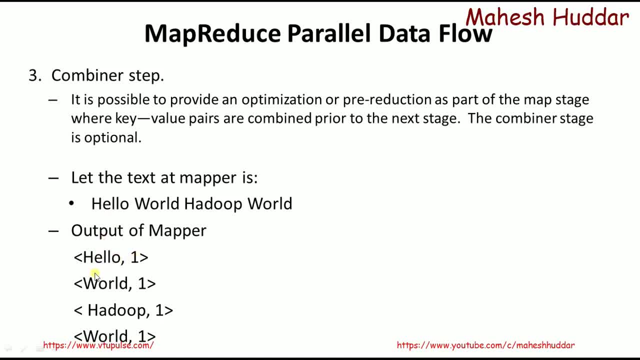 time. Hello is the first word, So it will take hello one is the output, So it comes across the second word. So world one will be the second output. Hadoop one will be the third output. World one will be the fourth output. Now, this is the only. 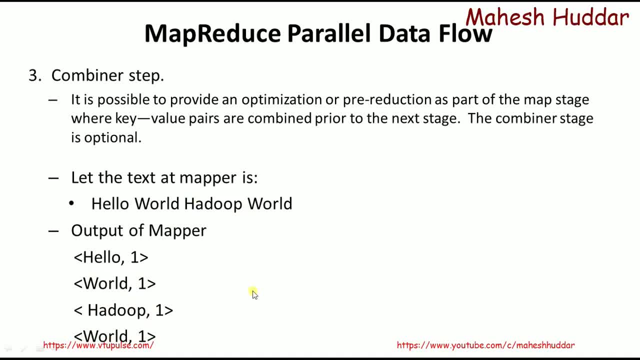 task done by the mapper. Now, what combiner does is in this output, that is, the output of mapper contains. some outputs are having the similar keys. So rather than giving this one as an input to the reducer or the next step, what it does is it will combine those results and it will create the 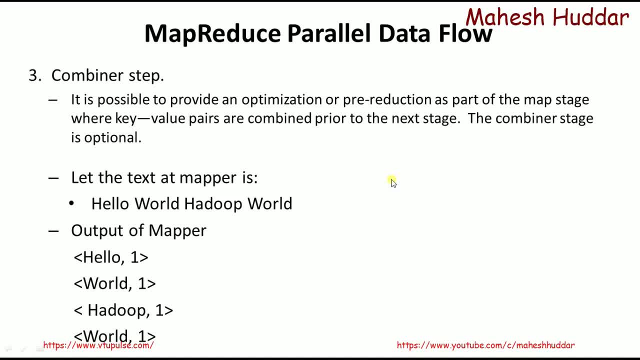 combined result something like this. So the output of combiner is: the hello is appearing one time, So there will not be any issue over here, but the world is appearing two times. So rather than passing this result two times to the next stage, combine it and get the. 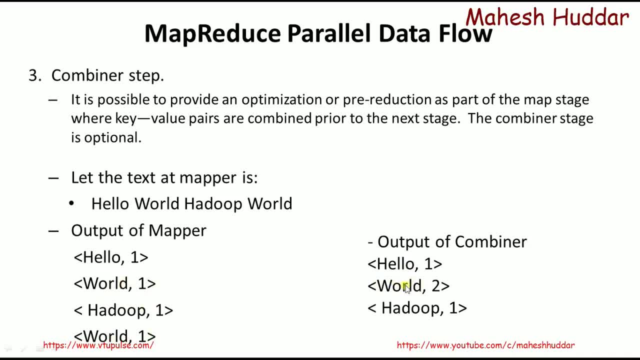 result in the form of key and value pair. Key will be, in this case, world and value will be two, because world is appearing two times. They add the values of the keys. So that is what actually has been done here. Next, the Hadoop is appearing one time. It will be as it is. So this is how. 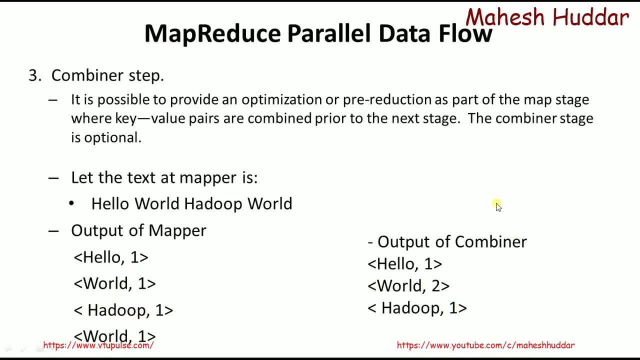 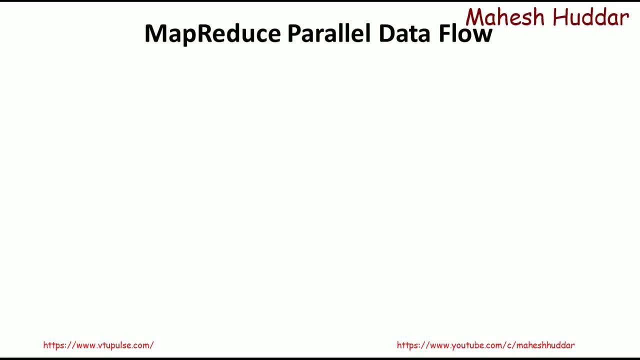 we will do some processing and the next processing will be done by the combiner and the combiner steps output will be given as an input to shuffle step. What shuffle step does is, if you see this particular thing, in this particular example, we have two persons. It is nothing but two mappers. 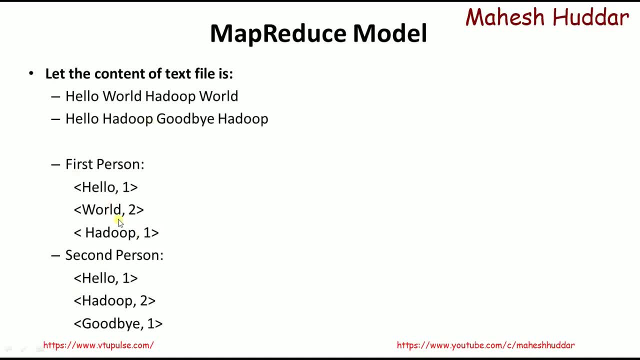 are present and the mappers are. two mapper programs have created some result output. The first mapper created an output of hello one, world two mapper, as well as combiner, that is, hello one, world two and Hadoop one. The second mapper has created hello one, Hadoop two and goodbye one. Let us 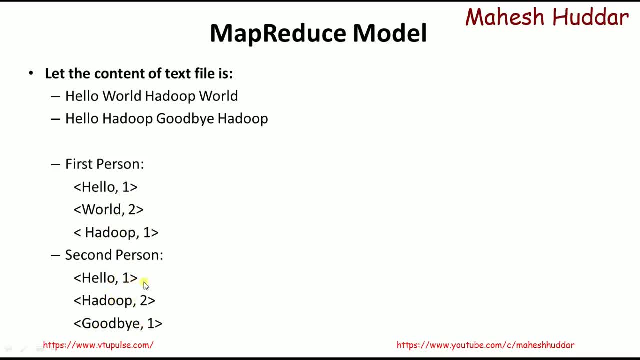 assume that this is the result. Now, what happens in shuffle step is it will take the output from both the mappers in this case, and then it will check whether it will come create a groups, groups depending on the keys. So now, here there is a mapper program and it will take the output. 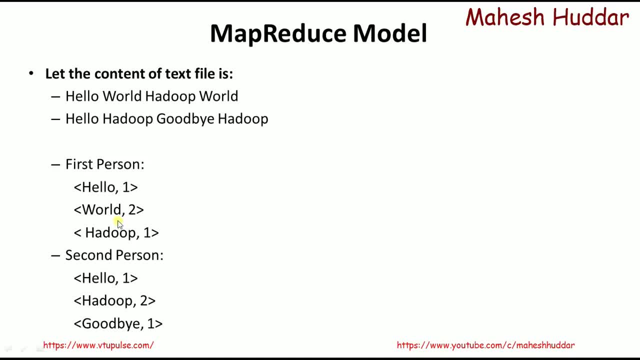 from both the mappers. There is an output called as hello one. There is an output called as hello one, because the keys are same. It will be in one group. There is a something called as world two. in this case. There is no world two here, and this will become another group. There is something. 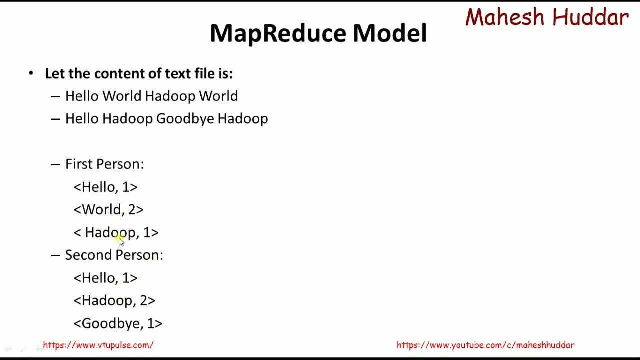 called as Hadoop one and Hadoop two in both these cases. So this will be the third group. in this case, The fourth group will become goodbye one. So that is the fourth group. So this is how actually the shuffle step does. What it does is it will combine the results of the mapper program with 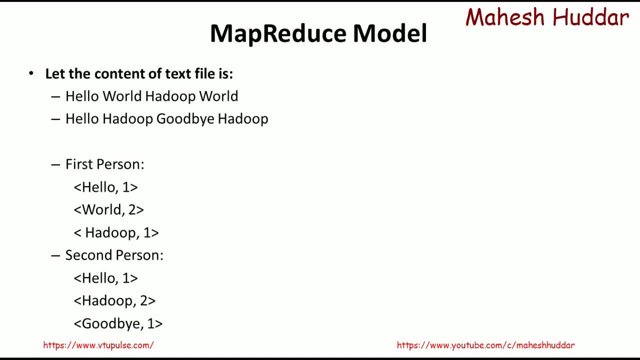 mapper and combiner into different groups depending on the key values. So in this case there will be four groups: Hello one, hello one, that is the first group. World two, that is the second group. Hadoop one, Hadoop two will be the third group. Goodbye one will be the fourth group. 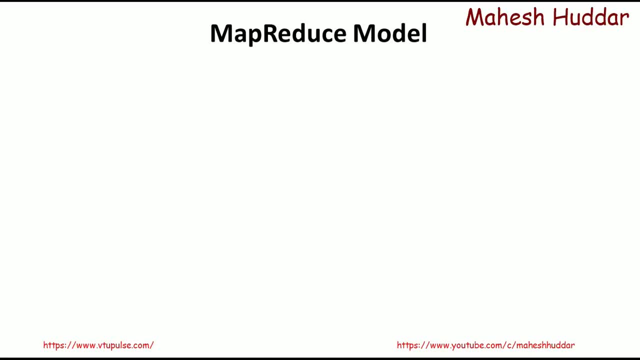 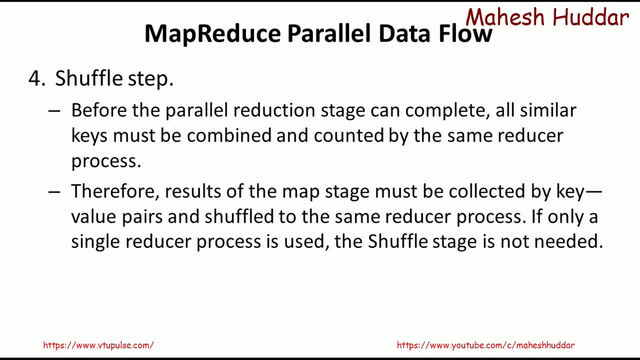 in this case. So that is what the output of this shuffle step- Now the output of shuffle- will be given as an input to the reducer step. What reducer step will do In the first group? as I told you earlier, there were four groups are there. The first group contains: 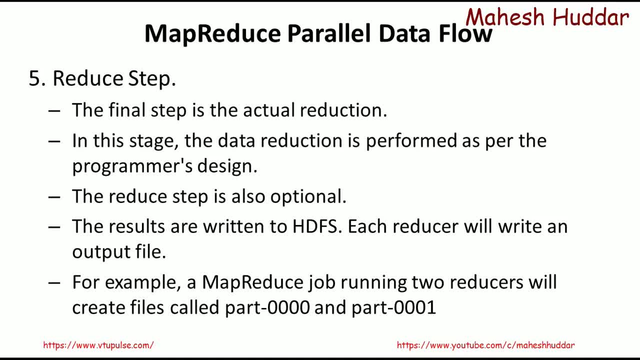 you can say that hello one, hello one. So what the reducer step will do? It will add: because this particular group has the key is hello, The output of this particular reducer step will be, the key will be hello and the value of this one is the values of both the outputs, that is, one plus one. 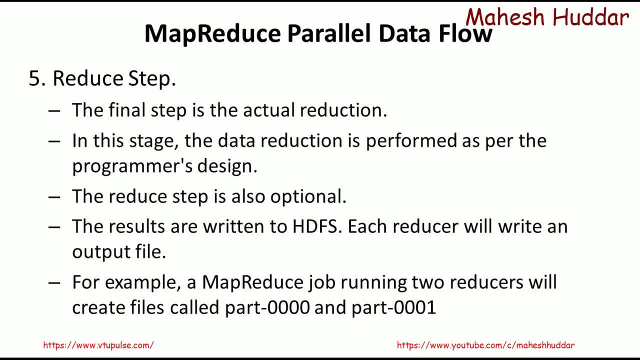 two. in this case, The second step was world two, because there is only one thing: World will be, the key value will be two and the output of the third group is actually. you can say that the third group is actually this one, that is, Hadoop one, Hadoop two, in this case, This particular. 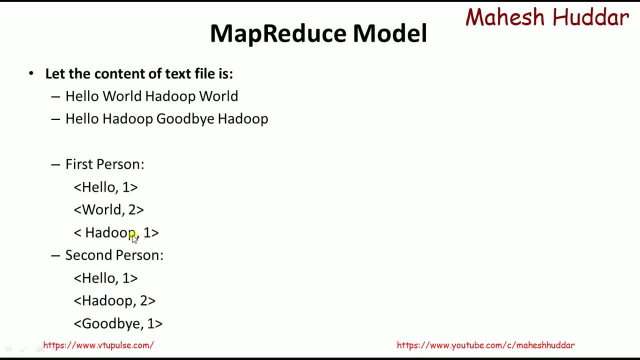 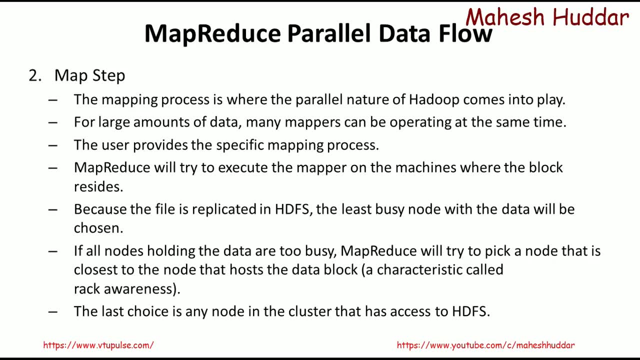 thing will be. the key will be Hadoop in this case, and the value will be, in this case, one plus two, that is, three in this case. So this is how actually the reducer will work and it will give you the final result. Depending on the number of reducers, it will generate different number of output files. So in 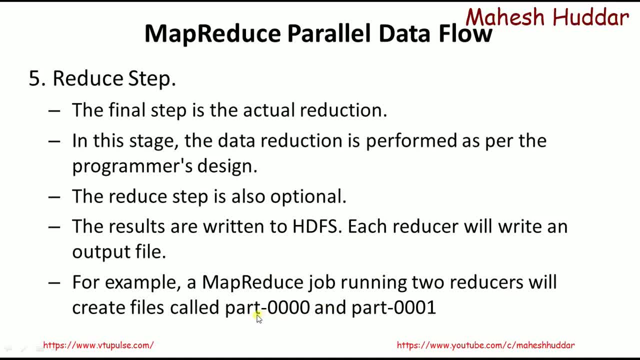 that example. I told you four reducers are there. definitely four outputs will be there. Just for example, assume that there are two reducers are there? the output will. output file will look something like this: one Part minus four zeros. Second, one will be part minus three zeros followed. 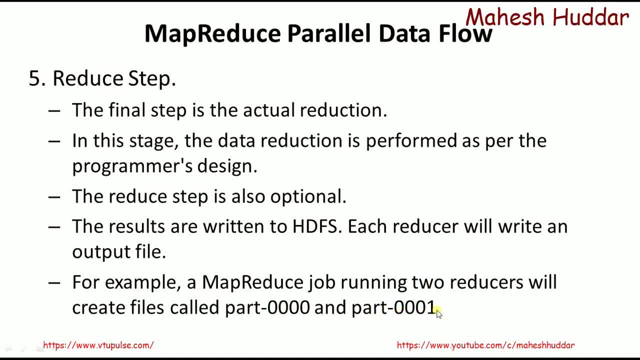 by one. If there is one more reducer, part minus zero zero zero two. If there is one more reducer, it will be part minus zero zero zero two, and so on, Something like that. the output file will be generated. The first output file will be related to one. 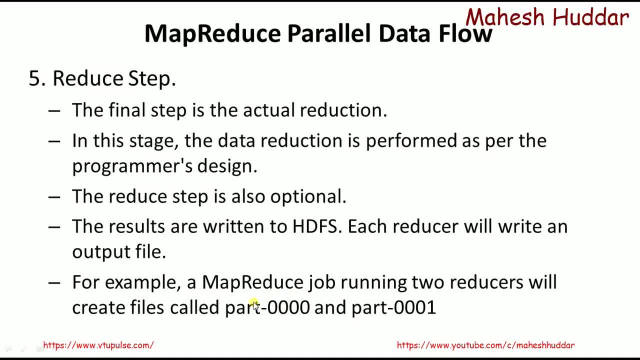 set of results. Second output file will be related to another set of results. So this is how actually the five steps of Hadoop MapReduce model works. Now we will go to the entire picture to understand the data flow in Hadoop MapReduce model. 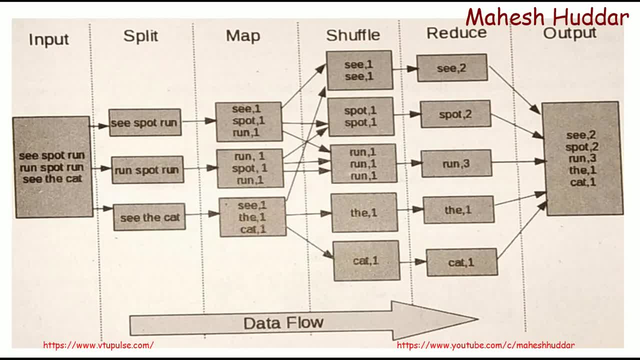 So initially there will be an input. As I told you earlier, the input will be divided into different number of data blocks. So this input contains- just to understand, we have not divided into 64 MB or something. The input is divided into depending on the number of lines. In this case, the input contains three lines, So three lines. 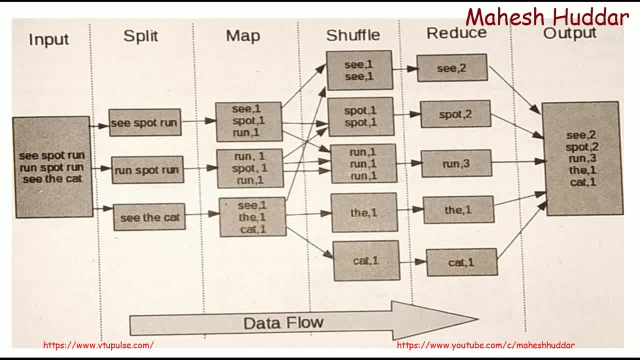 were divided into three. You can say that the groups- each group- will be stored into different data nodes. So that is how we can understand this particular concept. Now we will go to the next step Now, after this, this data is available on three data nodes, So mapper program will work on. 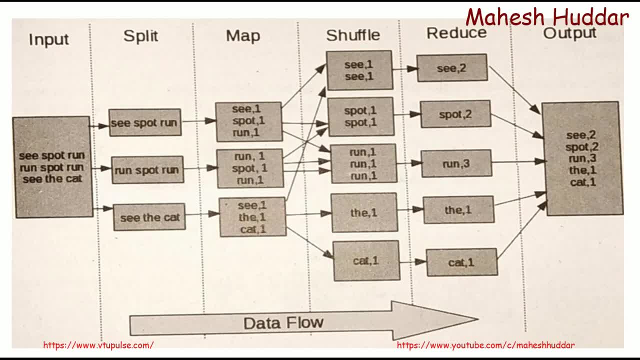 three data nodes. So first mapper program will run on. the mapper program will run on a data node one, data node two, data node three, because the data is available on three different data nodes. So what mapper does is it will create a key and value pair as 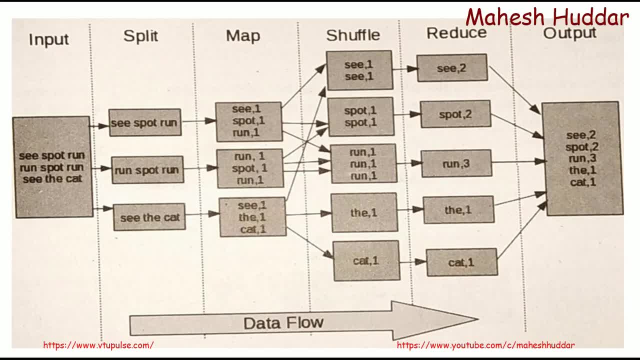 the output. It will check, it will read each and every word from that particular line and it will create an output where key will be the word and value will be one in this case. So the same thing will happen with respect to the second data node, The same thing will happen at the third. 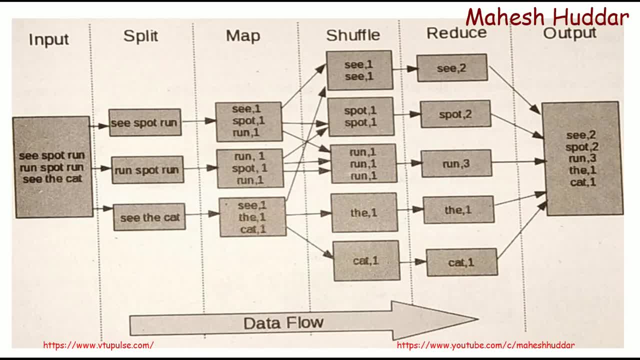 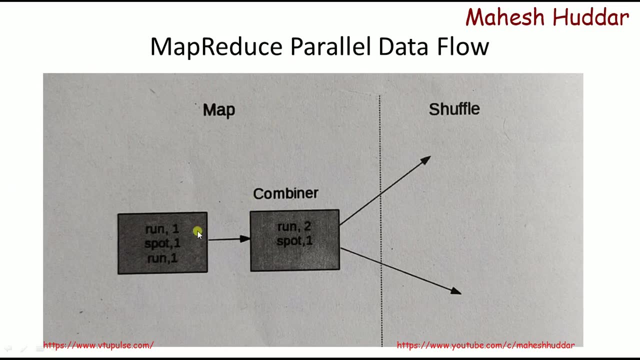 data node also. So the output of each data node looks something like this. Now, in this case the combiner is not shown. If combiner is shown, it will be something like this: In the second stage, second mapper, there is run is appearing two times. So 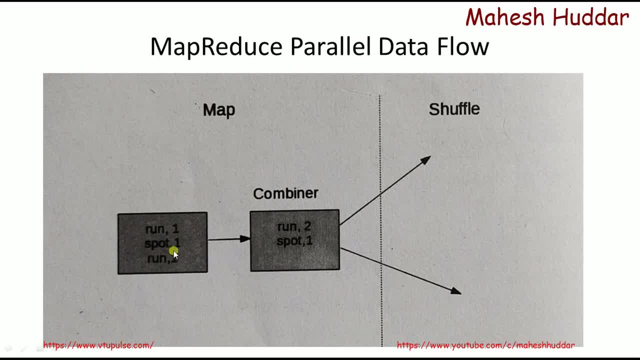 rather than giving these two outputs, we can combine this result and then we can give this one, the one output, as an input to shuffle step. So that is the only intention of having combiner stage. So in this case it was avoided because it is an optional stage. It may or 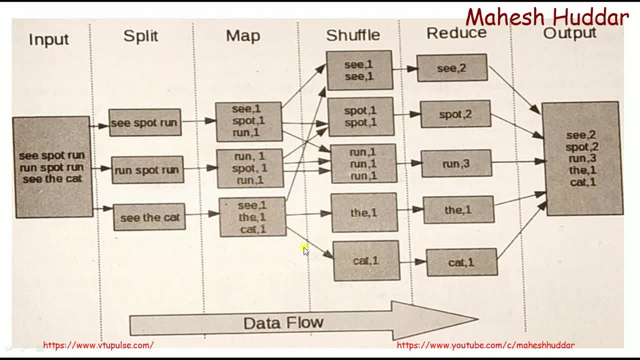 may not be available in the final model. Now this output is given as an input to shuffle What shuffle does, depending on the keys, it will group this particular results. So if you see this particular results, There is a word called as c in first mapper output as well as the c is present in the third mapper. 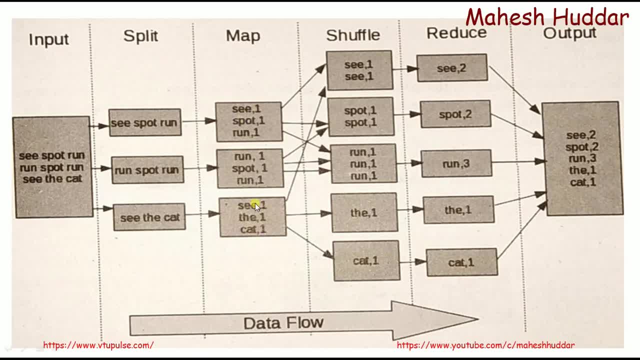 output. So these two things will be combined and it will be put into one group. The spot is present in first, the output of first mapper, and it is available in the output of second mapper. They will be grouped and it will be put into second group And similarly there will be a run group. 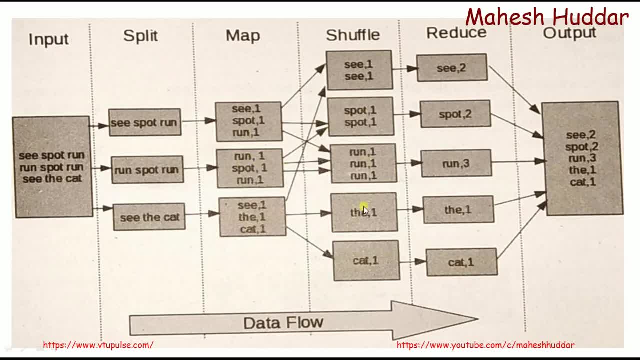 There will be a group for the word and there will be another group for cat word Now. so what shuffle does? depending on the keys, it will create a groups. Now these will be given as an input to different reducers in this case. So there are five groups are there? So there must be. 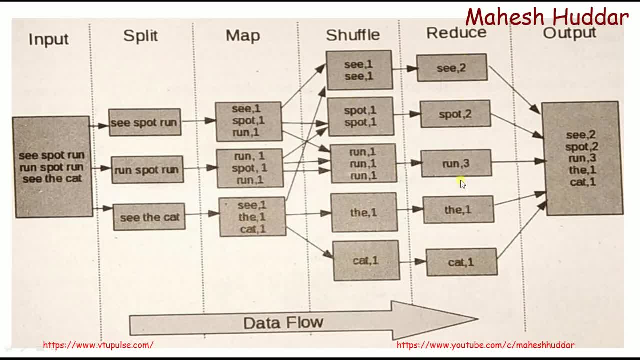 five, what we can say, that the reducers. So what the first reducer will do. The first reducer will take the result of shuffle as an input and it will add the values, because keys are same, in this case Keys what c that will become the key here also, and the value. 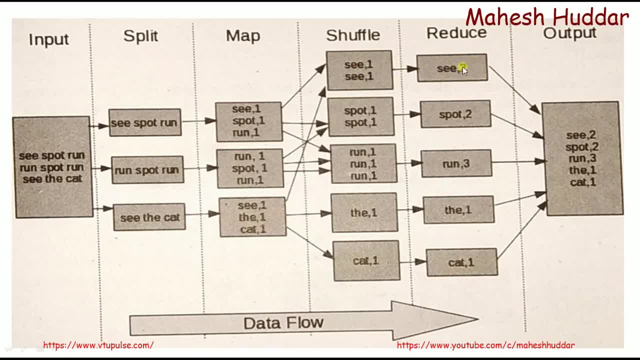 is So the sum of values of shuffle output. So that is in this case 2.. So spot will be the key 1 plus 1, will be 2 as the value. in this case, Run will be the key 1 plus 1 plus 1. that. 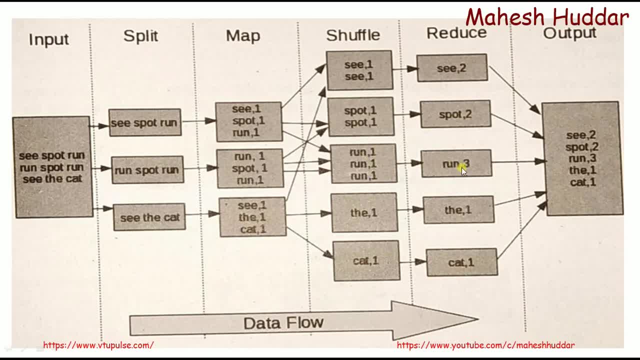 is 3 will be the value, and so on for the and cat words. So once this particular output is generated, it will be emitted as an the final output of Hadoop MapReduce model. So this is how actually Hadoop MapReduce model works. 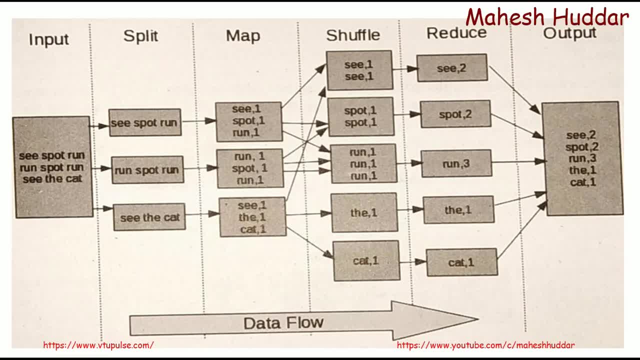 In this video I have discussed the basic idea behind the Hadoop MapReduce model. What are the different steps in Hadoop MapReduce model? with simple example, I have demonstrated how the data will flow from input to output in this video. I hope the concept is clear. 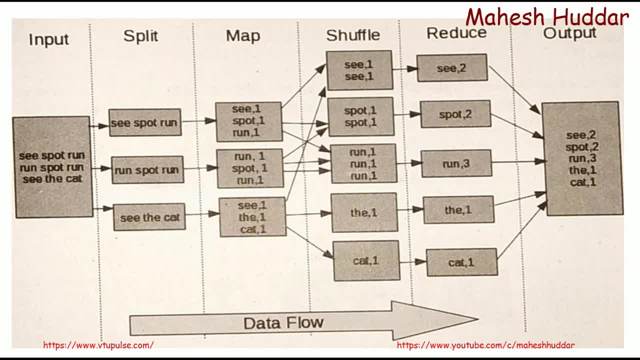 If you like the video, do like and share with your friends. Do subscribe the channel for more videos. Don't forget to press the bell icon for regular updates. Thank you for watching.